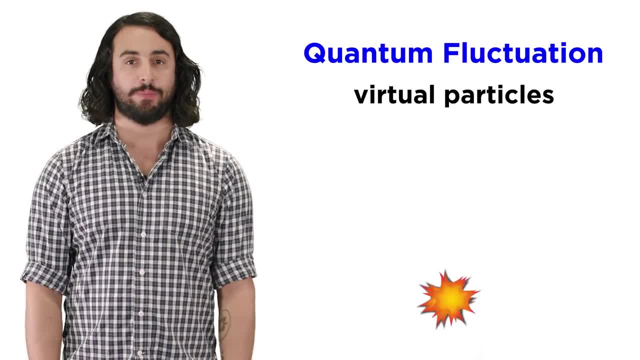 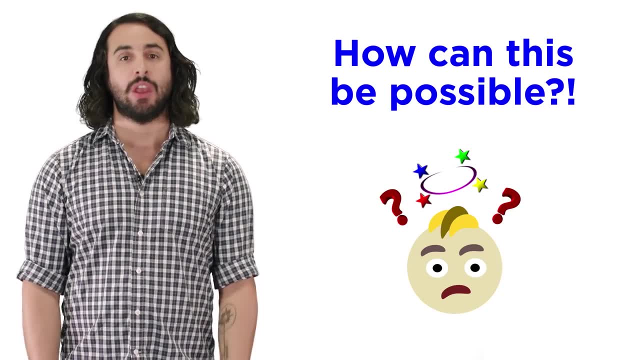 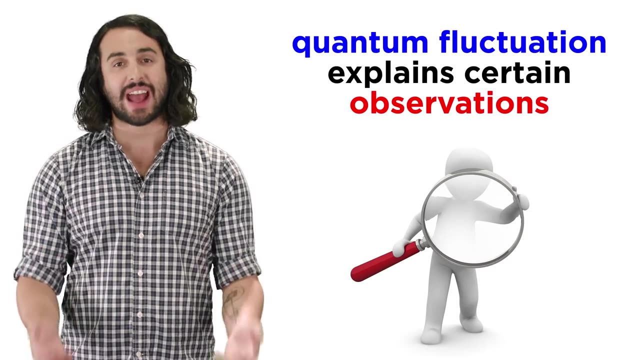 of time, We call these virtual particles, While it seems like this just can't be true, That it violates causality in everything we thought we knew about the universe. Quantum fluctuation of virtual particles is necessary to explain a number of observations, such as the Casimir effect. 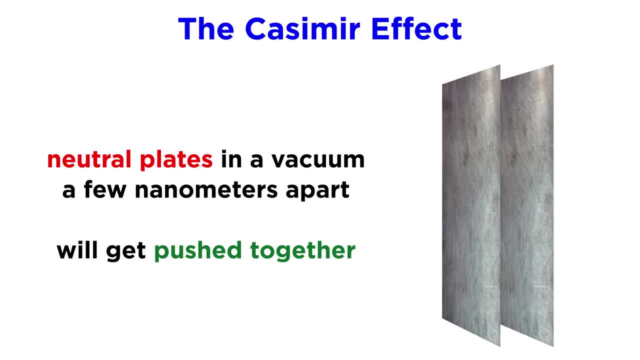 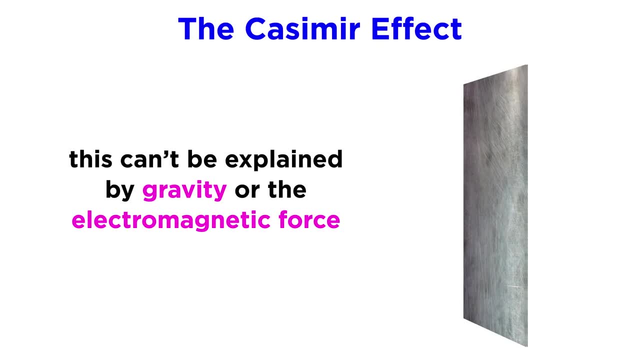 When two completely neutral plates are placed in a complete vacuum, just a tiny distance away from one another, they will eventually be pushed together. This can't be due to gravity or the electromagnetic force. instead, we must understand that there are more virtual particles coming together. 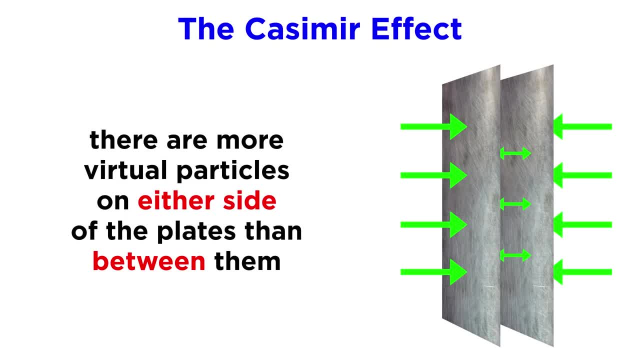 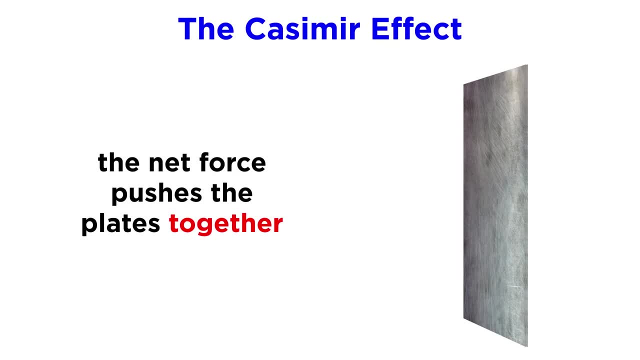 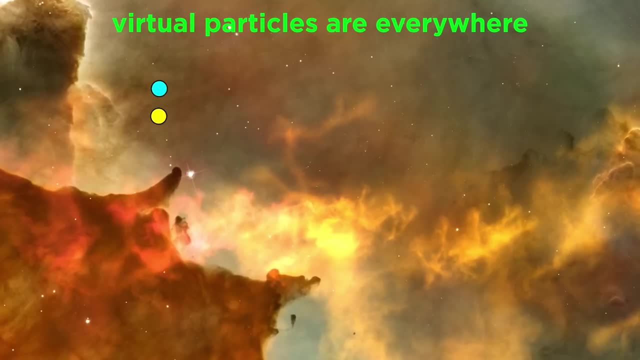 More virtual particles coming into existence on either side of the plates and imparting some force onto them than there are between the plates. so the net force pushes the plates together. Virtual particles arise all the time, everywhere in the universe, subsisting on borrowed energy. 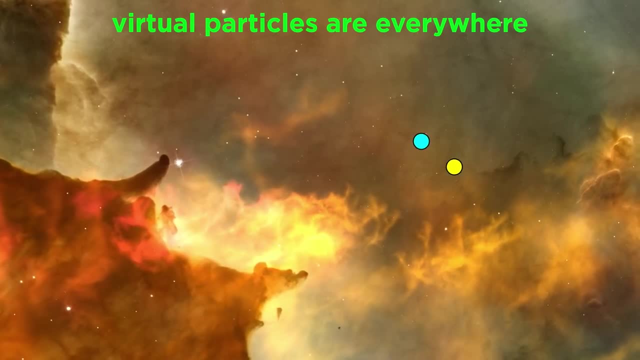 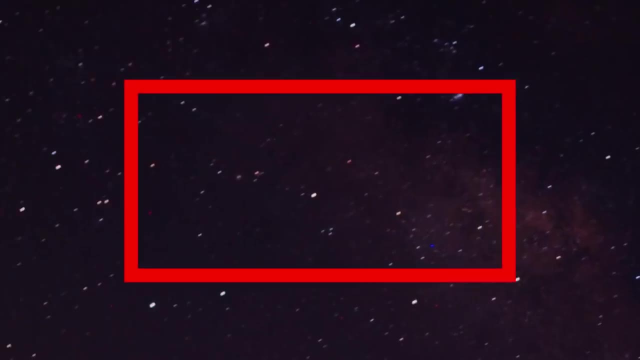 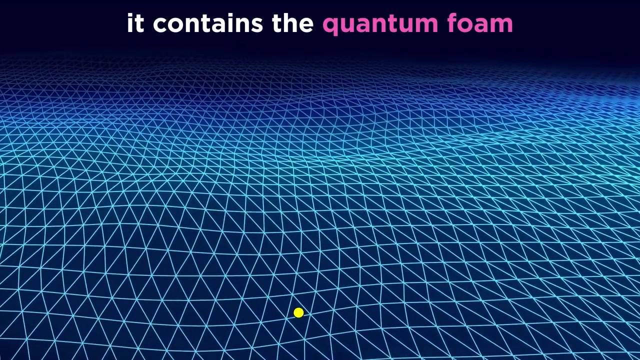 that is returned when they annihilate a tiny fraction of a second later. Through this phenomenon, we realized that empty space is not empty at all. It is actual substance unto itself. We call this property of space, the quantum foam, a sea of probability from which virtual 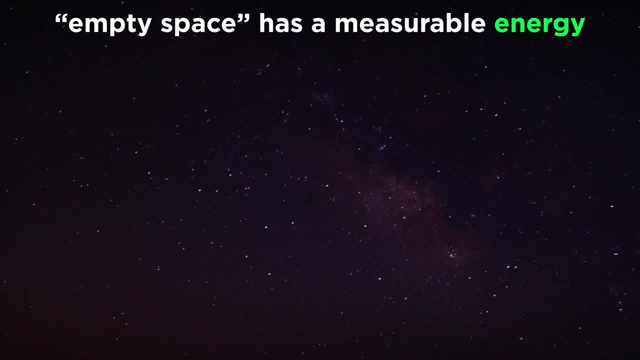 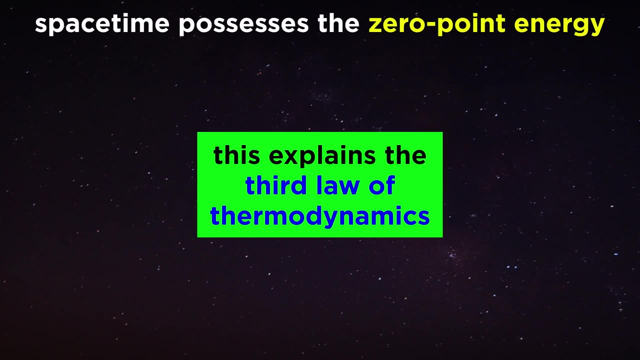 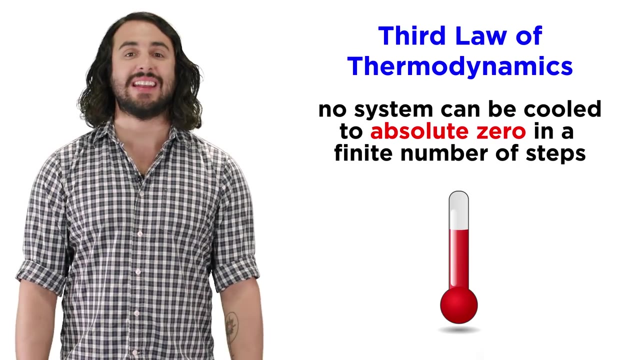 particles manifest and froth Because of this empty space actually has measurable energy. This is called the zero-point energy and it sheds some additional light on the third law of thermodynamics. In classical physics we understood that any system, including the universe, can never 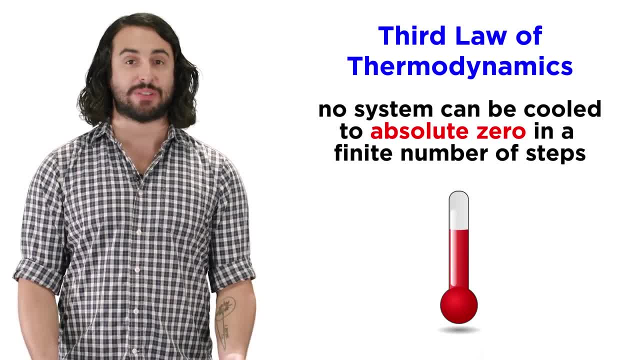 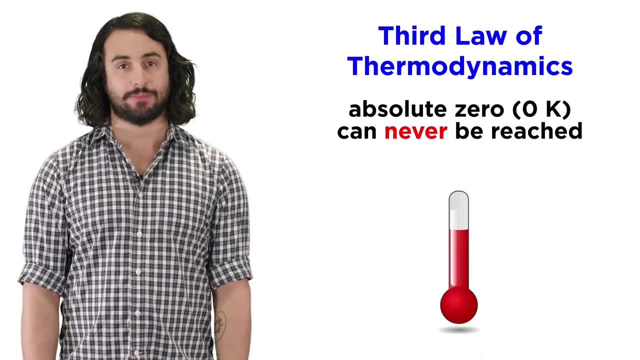 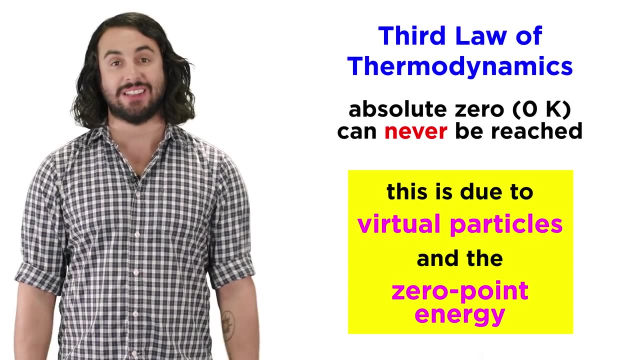 be cooled to absolute zero in a finite number of steps, Essentially meaning that absolute zero, a complete absence of kinetic energy, can't be reached. Now we know why: Because there will always be the tiny amount of energy irrevocably contained by space itself. 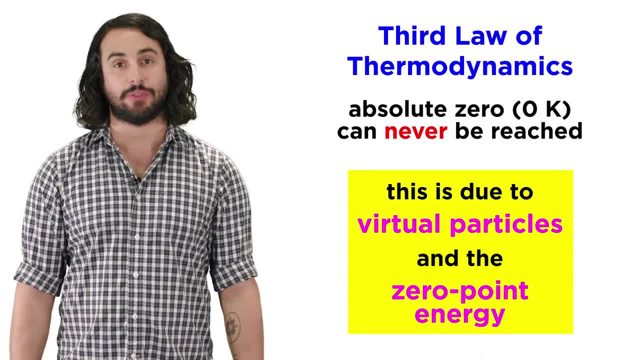 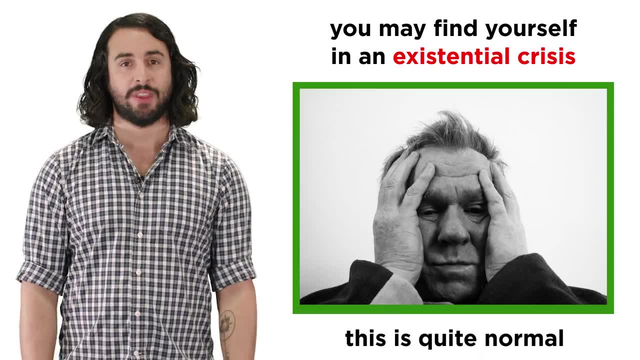 preventing us from peeling away those last few thousandths of a kelvin. By now, you should feel sufficiently confused, possibly on the brink of existential crisis. If this isn't the case, you may not have been paying attention. I hope you enjoyed this video. 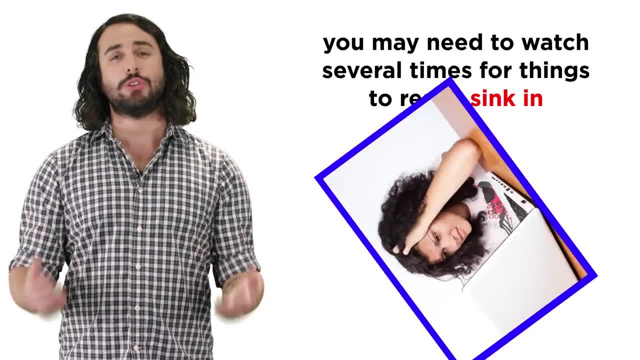 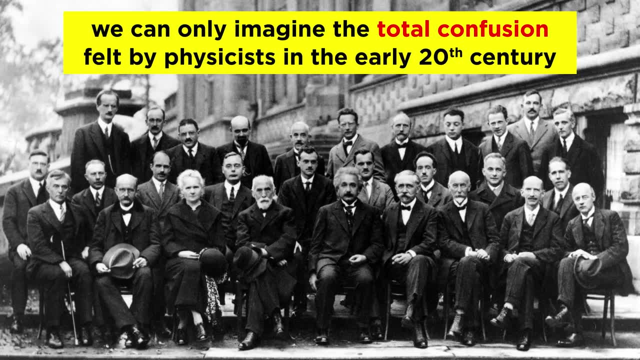 Thank you for your attention, so you'd better go back and watch again If you do indeed feel reality spinning away from you. congratulations, you have a small window of insight into how it felt to be a physicist in the early 20th century.